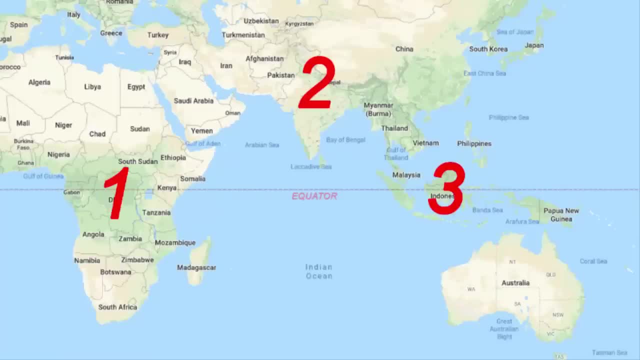 If you look at the Indian Ocean, it is surrounded by land masses on three sides, But on the eastern side water from the Pacific flows between the islands of Indonesia and Australia and mixes with the Indian Ocean. The tropical easterlies make that happen. 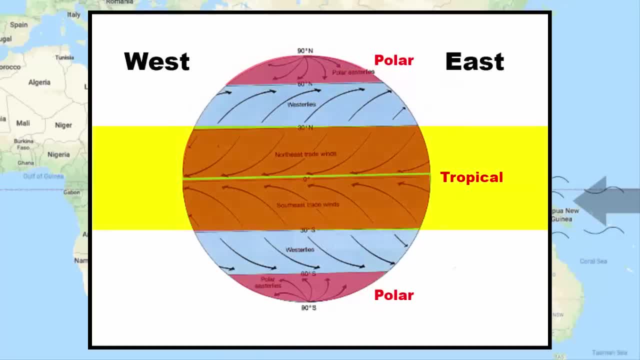 Tropical Easterlies are winds that blow from the north-east in the northern hemisphere and from south-east in the southern hemisphere, and they are located between 0 and 30 ° north and south latitude. When the water from the Pacific Ocean moves into the Indian Ocean, it changes the surface temperature of the Indian. 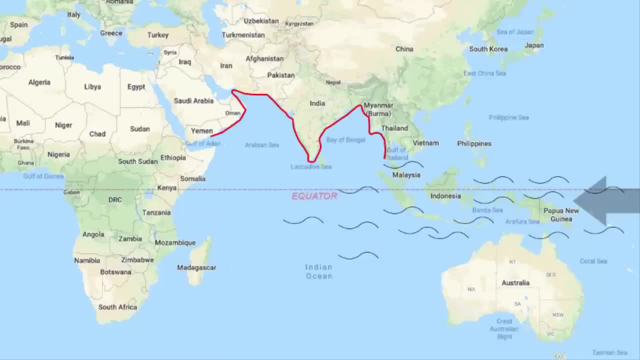 Ocean water. Another fact is that in the Northern Hemisphere the Indian Ocean is landlocked and doesn't come in contact with the Arctic waters. That means the water of the Indian Ocean is pretty much warm all throughout the year. So these are some of the reasons as to why the Indian Ocean 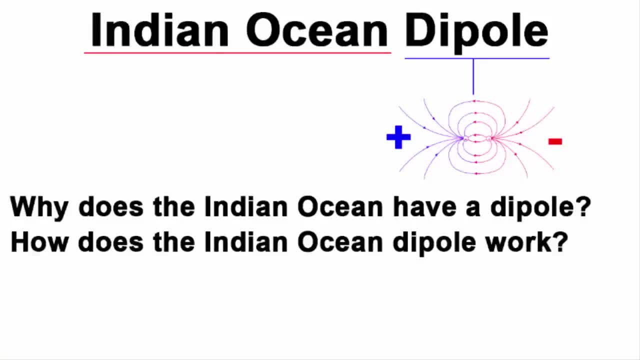 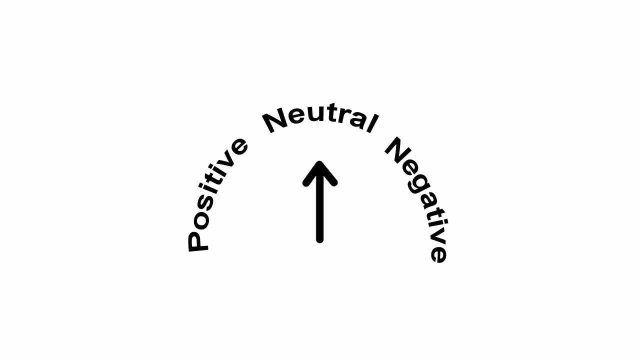 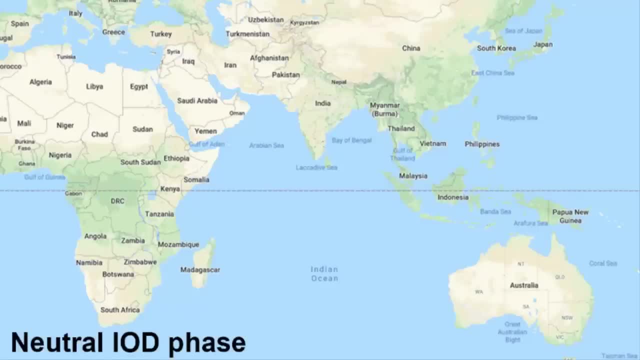 develops a dipole. Now let's go to the next question: How does the Indian Ocean dipole work? The Indian Ocean dipole varies between three phases: neutral phase, negative phase and positive phase. First we'll look at the neutral IOD phase. The neutral phase begins during spring season, when 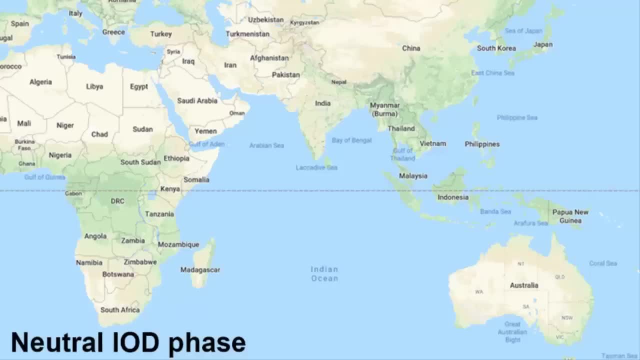 temperature gradually rises During the neutral phase. the water from the Pacific flows between the islands of Indonesia and Australia and comes in contact with the Indian Ocean. Temperatures are close to normal across the Indian Ocean. Then comes the positive IOD phase. In this phase, 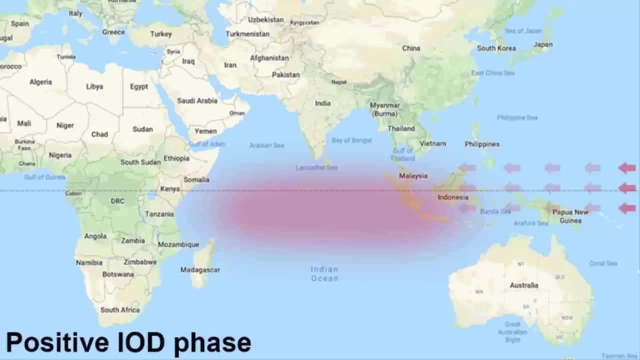 more and more warm water of the Pacific starts to flow between the islands of Indonesia and Australia. Now, keep in mind, there are strong tropical easterly winds that flow in this region. Now these strong tropical easterly winds push the warm surface water towards the western side of the. 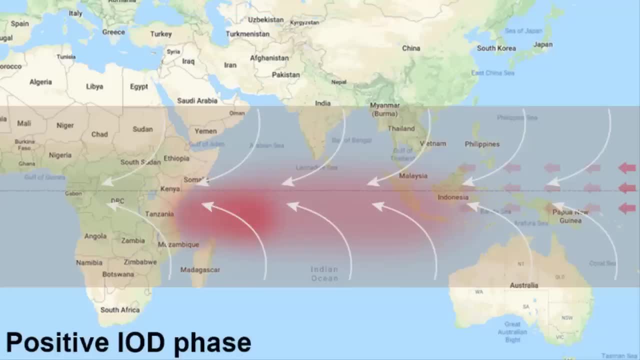 Indian Ocean that is near Africa. When that happens, you also have to pay attention to the thermocline. As the surface water is warm, the temperature of the water below the surface is cold When warm surface water accumulates on the western side. 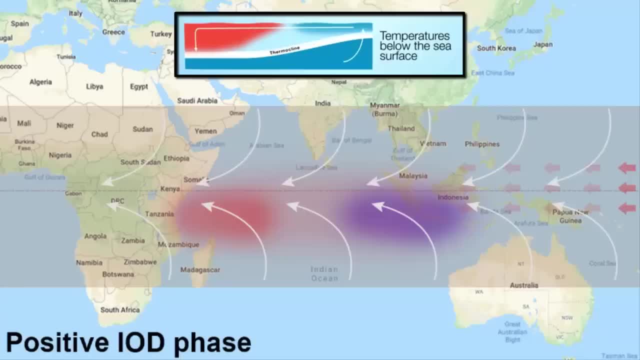 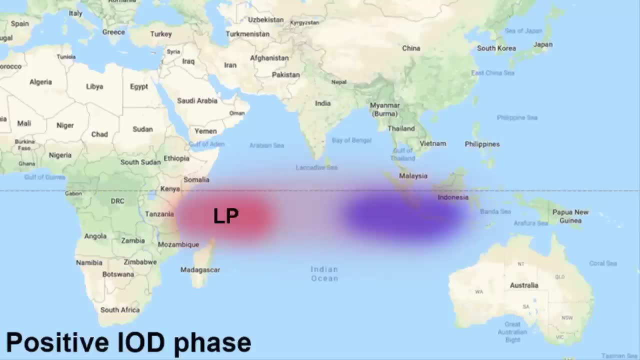 the temperature of the water below the surface is cold. When warm surface water accumulates on the eastern side, deep cold water rises towards the surface on the eastern side. This process is called upwelling. Now the warm surface water on the western side of the Indian Ocean will create a low-pressure. 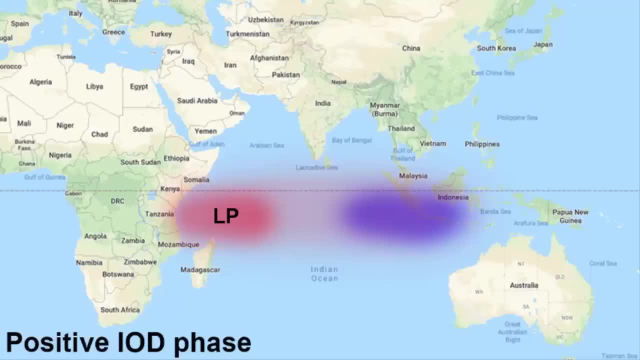 zone. Always remember: low pressure will develop in the region of warm temperature. Warm temperature also creates a lot of moisture. The warm air then rises because the hot air molecules are loose Air expands when it is warm. After reaching a certain height, some of the warm air condenses. 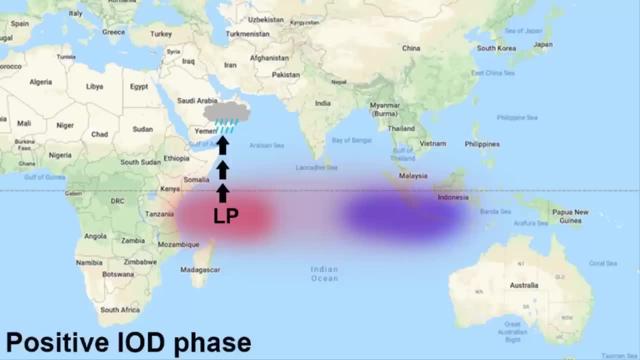 which then results in rainfall. On the eastern side of the Indian Ocean, you will find the ocean water to be cooler. Cold temperature is associated with high pressure. At high pressure region the air sinks because cool air is more dense and heavy. 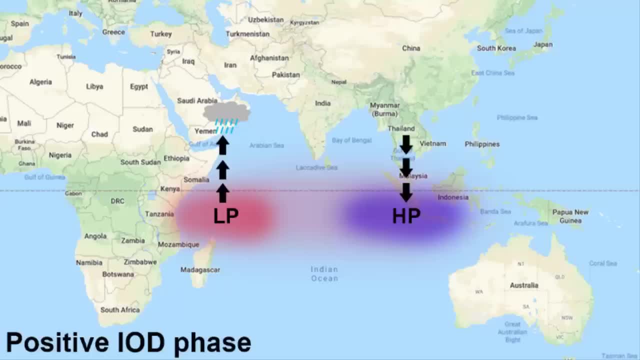 When cool air descends, it warms. Since it can then hold more moisture, the descending air will evaporate water on the ground. That's why the region of high pressure will usually have drier conditions. There will be no clouds and no rainfall. 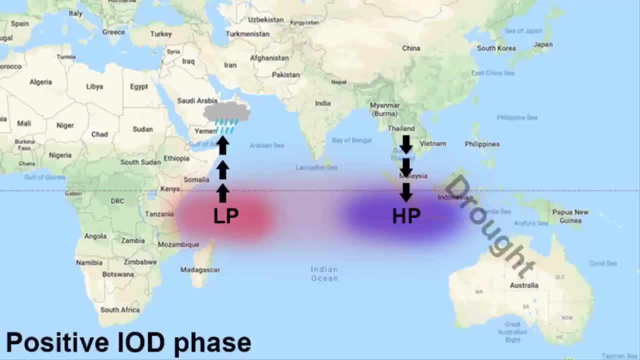 During this time, the southeastern countries and northwestern Australia faces severe drought conditions. On the other side, the coastline of Africa faces severe rain and floods. Air flows from high pressure to low pressure area. This is what creates the global wind belts that profoundly affect regional climate. 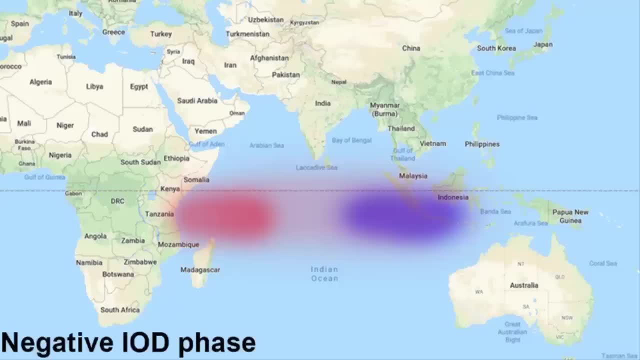 That's how the entire circulation of air occurs. And the third phase is the negative IOD phase. In this phase, the easterly winds become weak and the westerly winds become strong. The westerly winds push the warm surface water from the western side of the Indian. 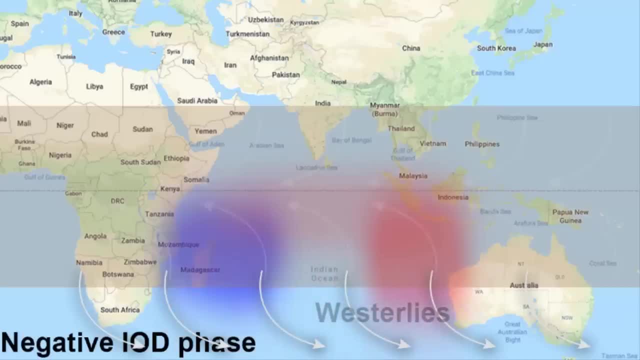 ocean towards the eastern side, that is, near Indonesia and Australia. When warm surface water accumulates on the eastern side, the deep cold water rises towards the surface on the western side. The warm surface water on the eastern side of the Indian ocean will create a low pressure. 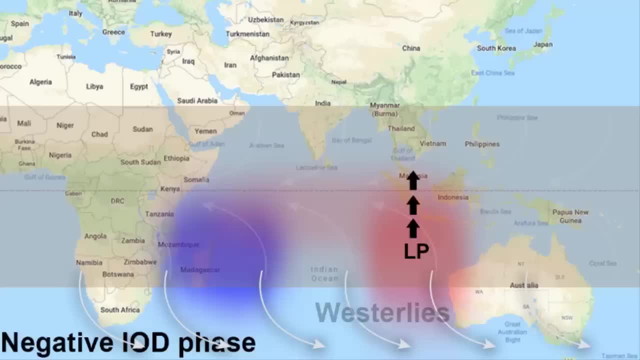 zone. The warm air will then rise because the hot air molecules are loose. Air expands when it is warm. After reaching a certain height, Some of the warm air condenses and form clouds, which then results in rainfall. On the western side of the Indian ocean, you will find the ocean surface water to be cooler. 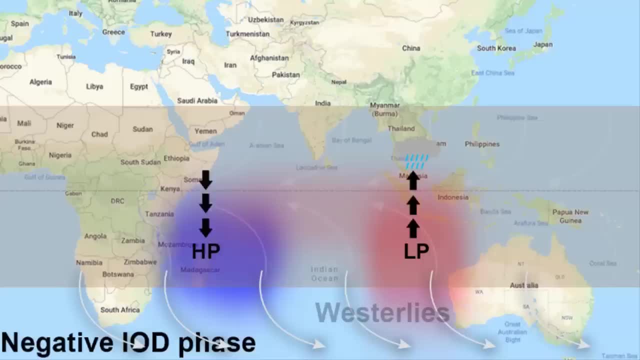 Cold temperature is associated with high pressure. At high pressure region the air sinks because cool air is more dense and heavy. During this time, the southeastern countries and north western Australia gets rain. On the other side, the coastline of Africa faces severe drought conditions.